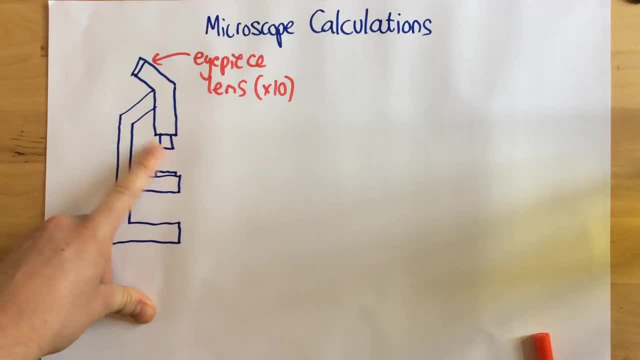 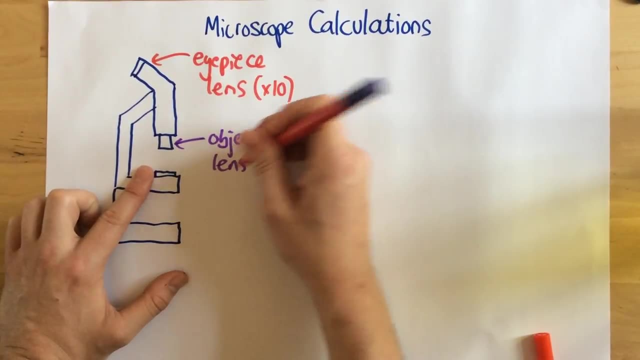 So we can help you read it. would you have an illusion of seeing 대聢 envision, Sean, But I don't. objective lens is this lower one here. it's the one that we use to look at the object, so that's why it's called objective lens. now, this one normally has. 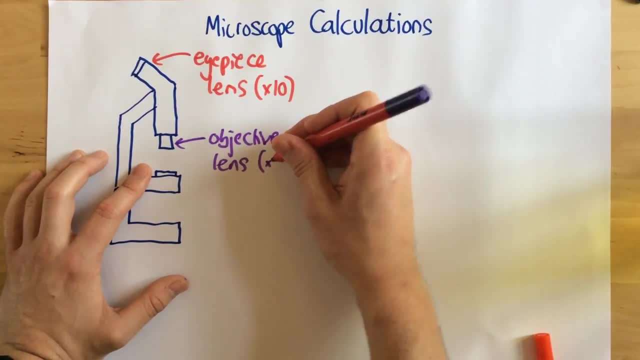 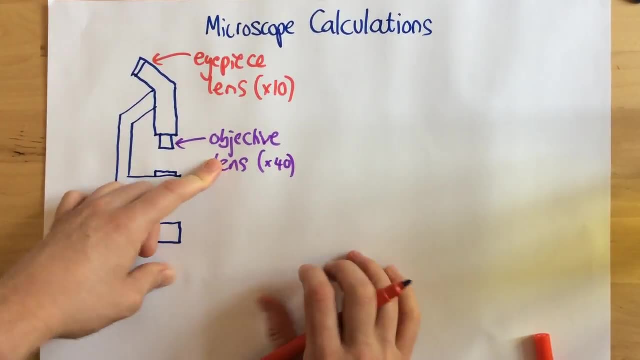 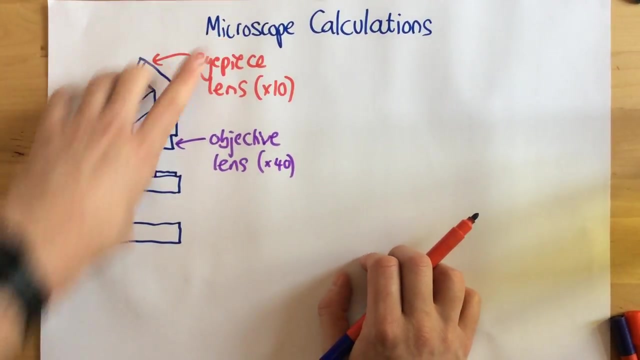 a higher magnification, the eyepiece lens. sometimes it would be maybe up to 40. now microscopes normally have more than one objective lens and you could actually change them round, but at any one time there's only one in use. so the first equation we need to know, or the first kind of bit of maths with microscopes- 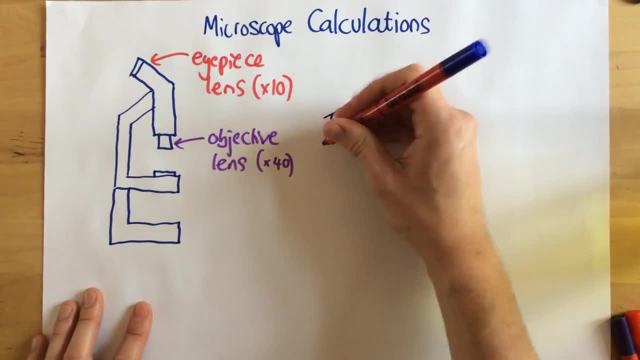 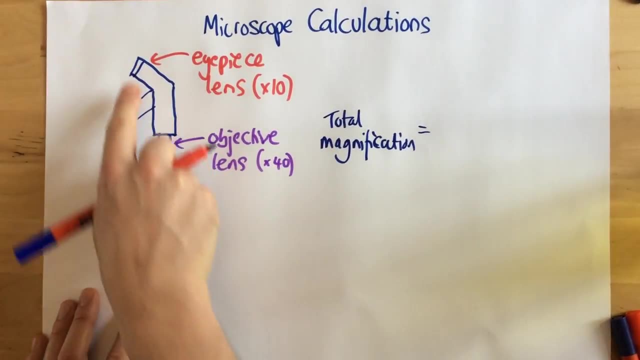 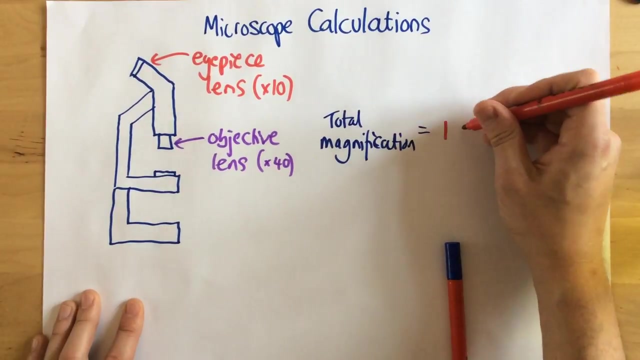 we need to know is really easy to find the total magnification. all that we need to do is multiply the two different lenses together, so the magnification strength of the two different lenses. so for this particular example of this microscope, I just need to take my magnification, my eyepiece lens, multiply. 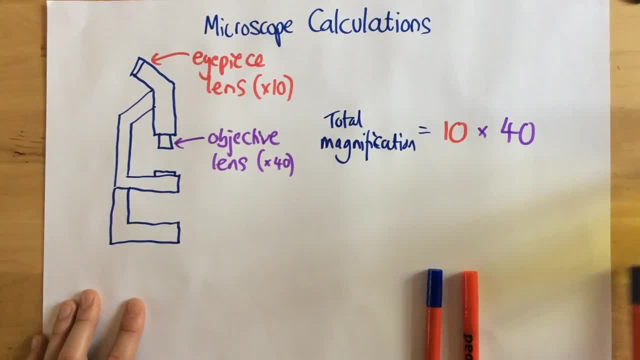 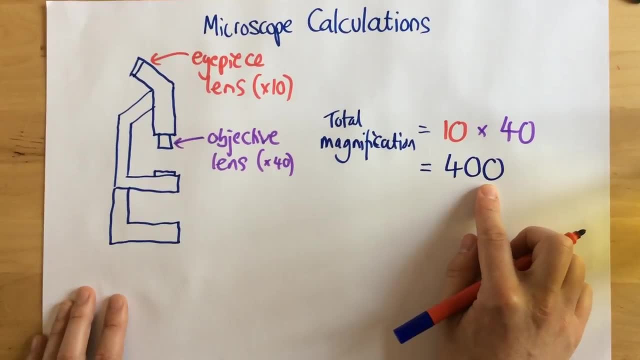 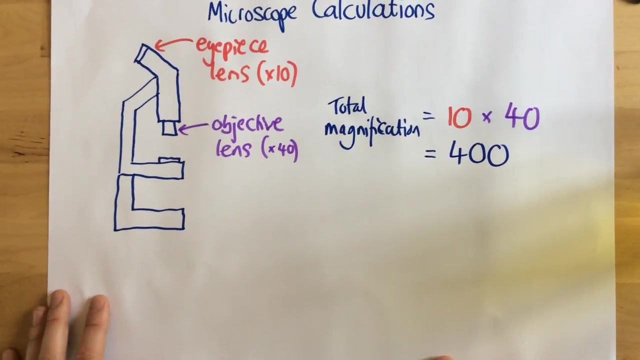 it by the magnification of the objective lens. and nice and simply, that is going to say that this microscope now is going to have a magnification of 400, so it means that image was going to appear 400 times bigger. really, really simple. now the next part of microscope: 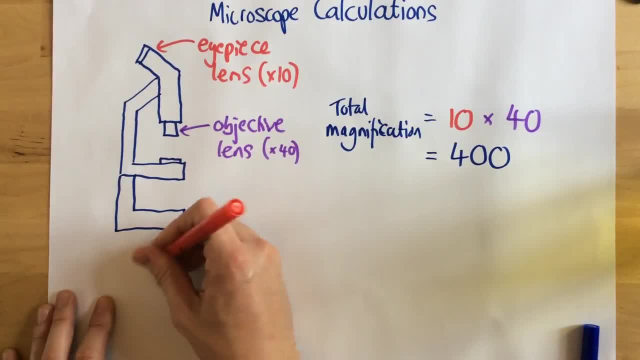 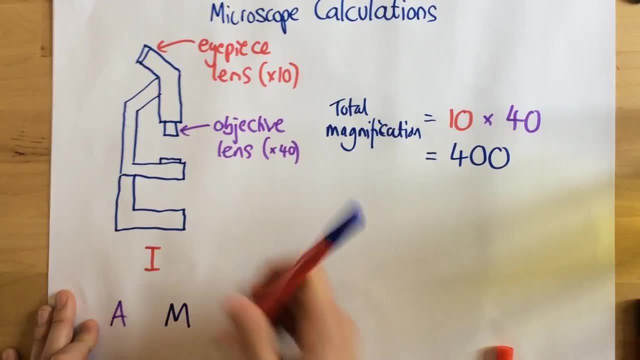 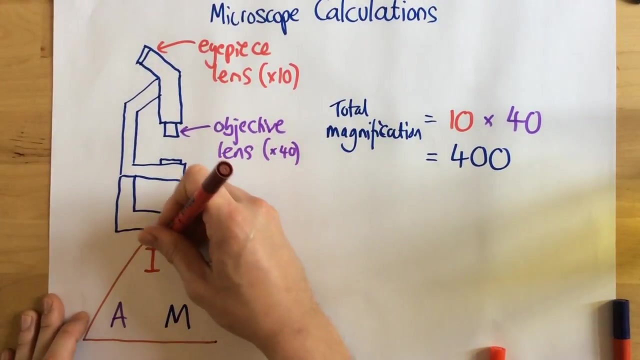 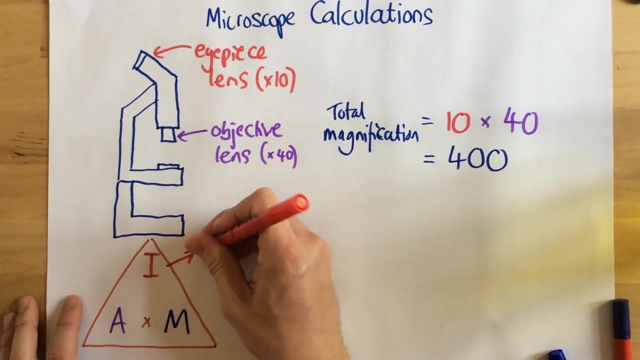 calculations that we need to know is this particular equation triangle. now, it's nice and easy to remember it because we can just remember this: I am, I am, I goes on top and I'm across the bottom, so we just read it from the top: I am. now. what this stands for is this: I stands for image size. now that, what that? 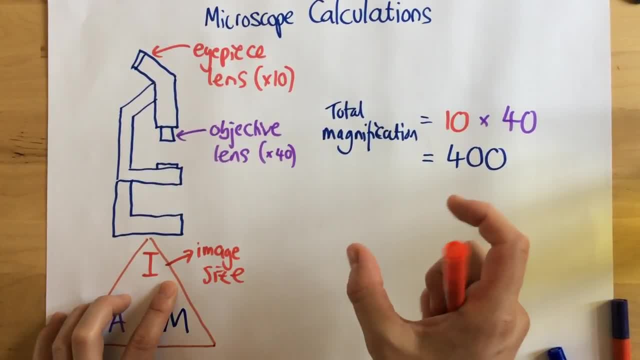 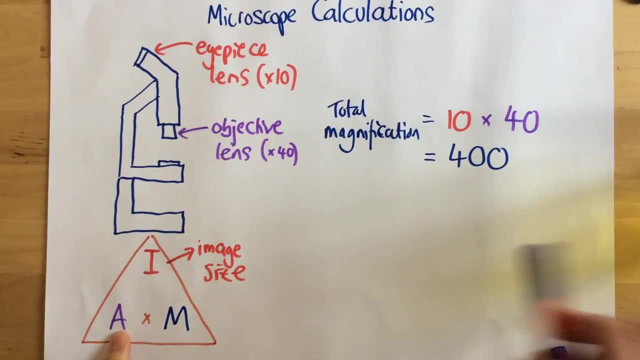 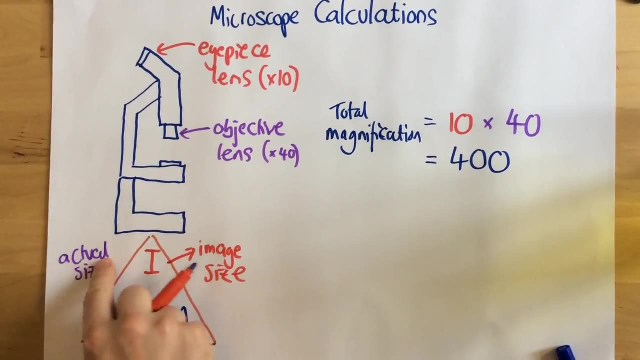 means is: how big is the image? that with, how big is the image once viewed? not how much. how big is it in real life? because a that stands for actual size. so this is how big that the thing is we're looking at in real life. And finally, 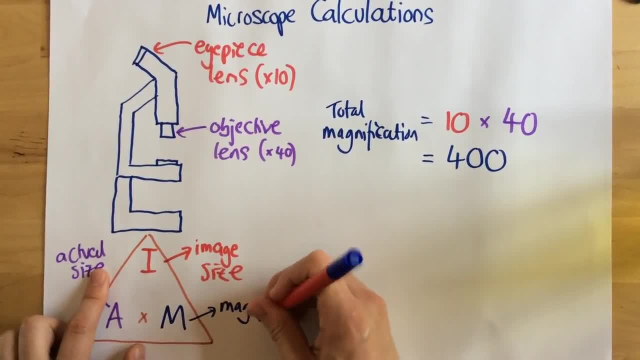 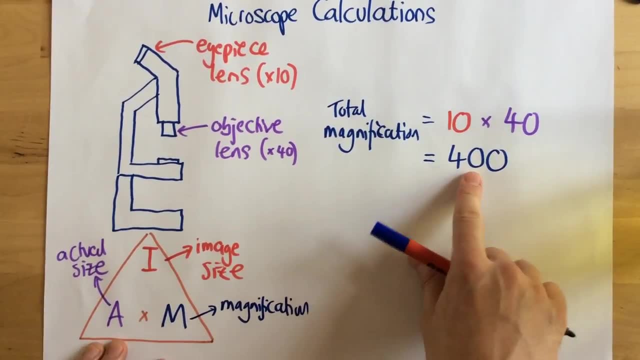 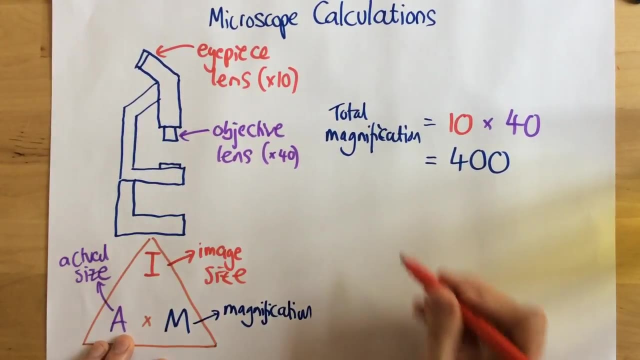 M stands for magnification. So what that means is: how many times is that image being magnified? How many times bigger is it? So let's have a quick example. let's see how this works. So let's imagine I've used my microscope and 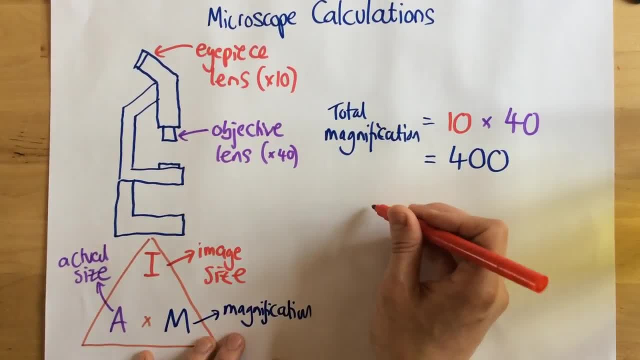 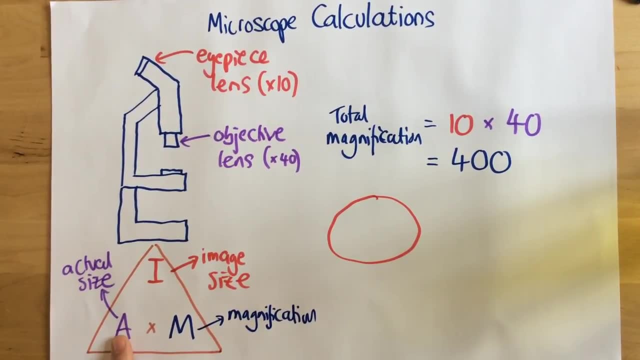 I've got myself an image which is this big here, so I'm just going to draw an image. Now what you might have to do is, let's say, we're trying to find how big this, this thing, and this could be a cell, for example, but how big. 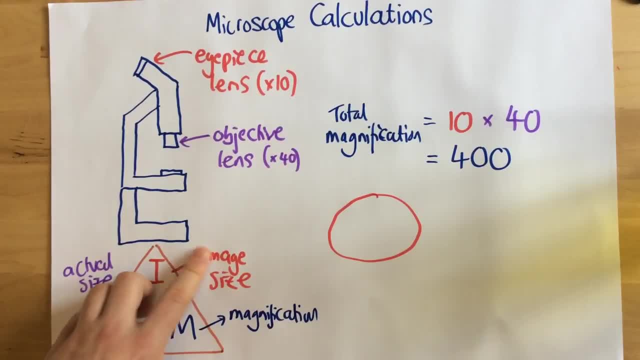 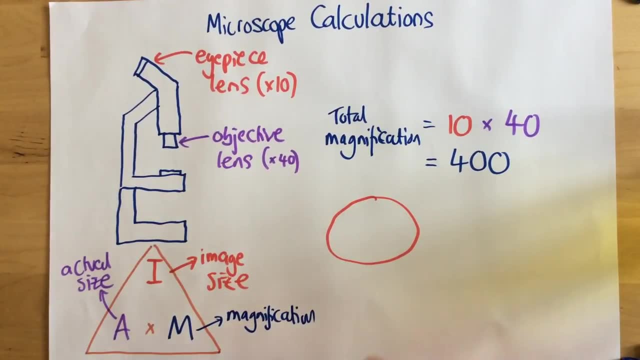 is this thing in real life. So what I've got here is the size of my image, and let's say, I'm using this microscope here, so that's my magnification. So the first thing I need to do is I need to see how big this image is, so I could just measure this with a ruler. 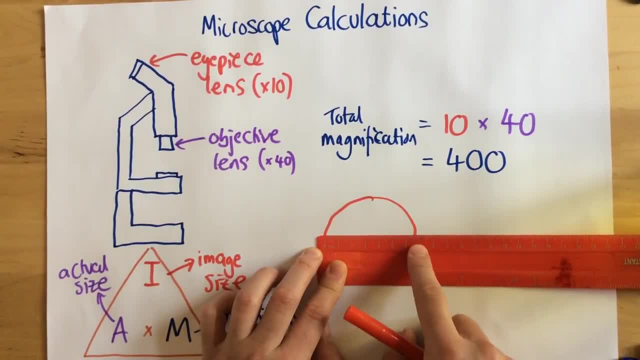 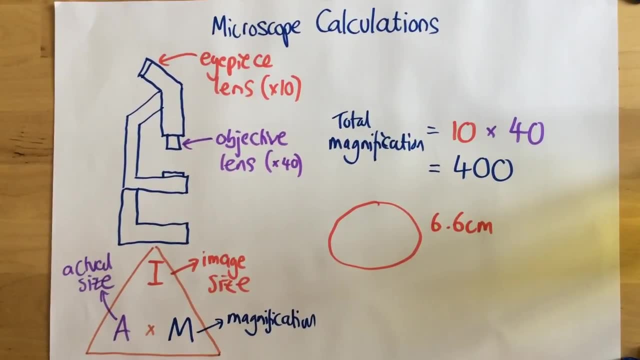 So this here is about 6.5 centimeters in diameter. So what I then need to do is I then need to use this equation triangle to find the actual size. So, just like normal, whenever I use an equation triangle, I cover the thing that I'm 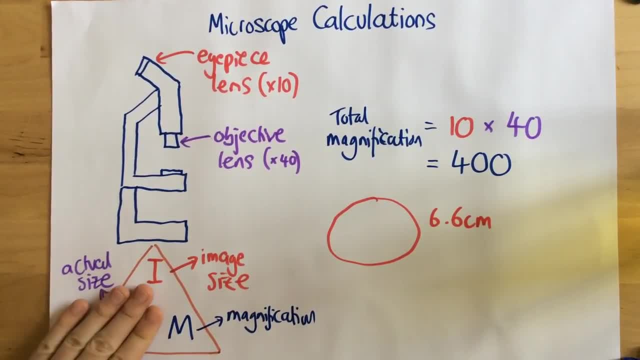 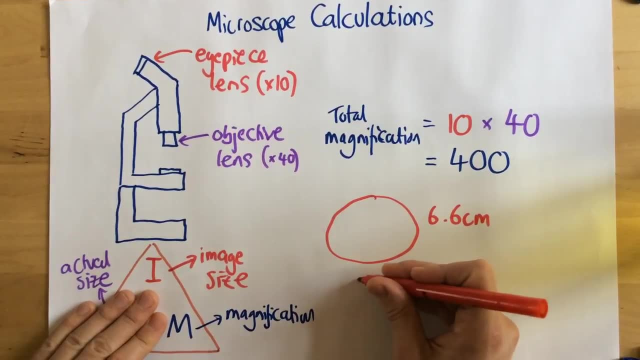 looking for. So I'm looking for the actual size, so I'm going to cover that up. So what I'm going to need to do is I'm going to need to take my image size, which is 6.6 centimeters. 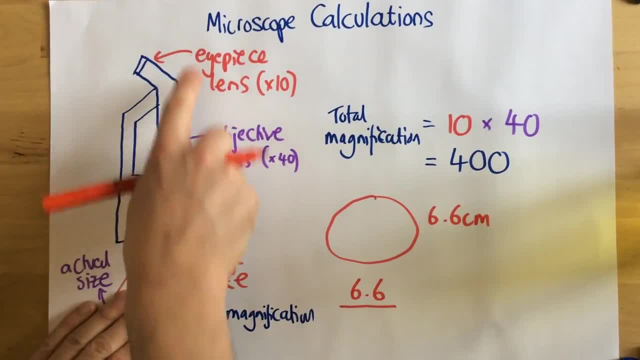 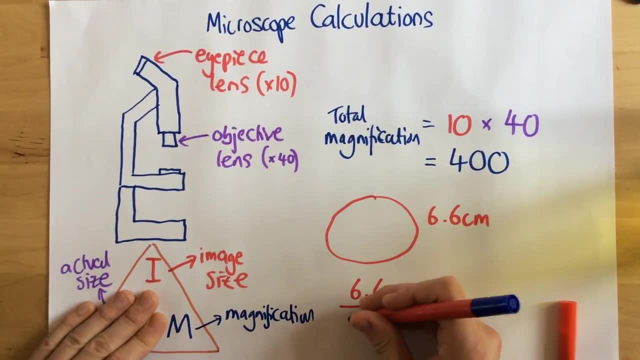 and divide it by the magnification For this particular microscope, remember, because the eyepiece lens is 10 and the objective lens is 40, the total magnification is 400.. So all I'm doing is 6.6 divided by 400. 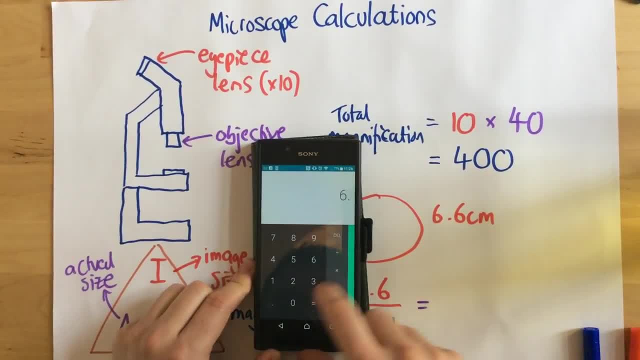 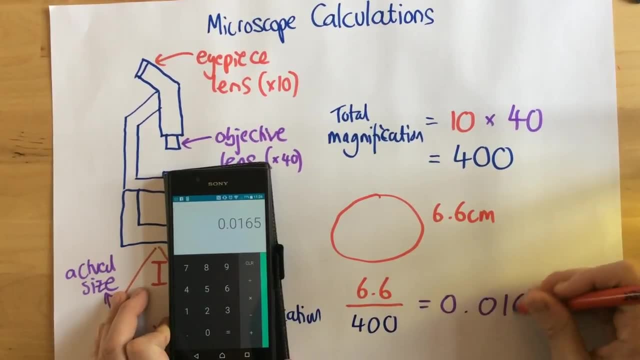 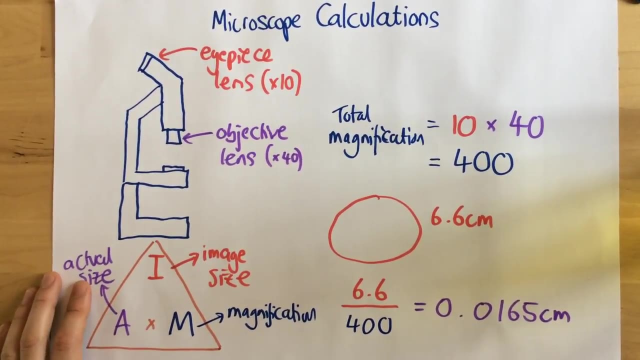 in order to find my actual size. So then, I just need to do this on a calculator: 6.6 divided by 400, which equals 0.0165 centimeters. Now, what they might ask you to do- probably ask you to do- is you might have to. 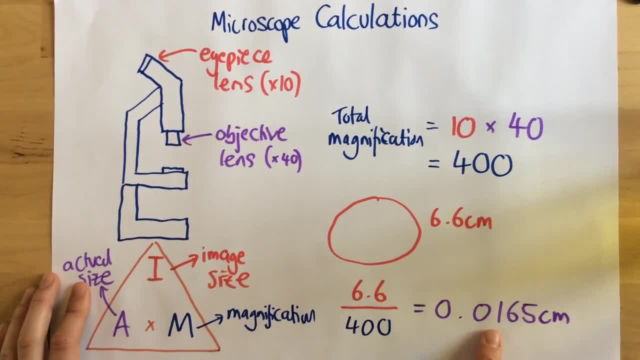 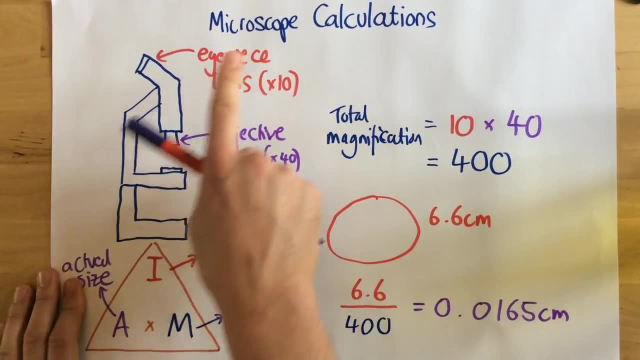 convert this to a different units, for example micrometers, But I'm going to show that in a different video. So just to summarise: to find the total magnification, you simply multiply the magnification of the eyepiece lens by the magnification of the objective lens. 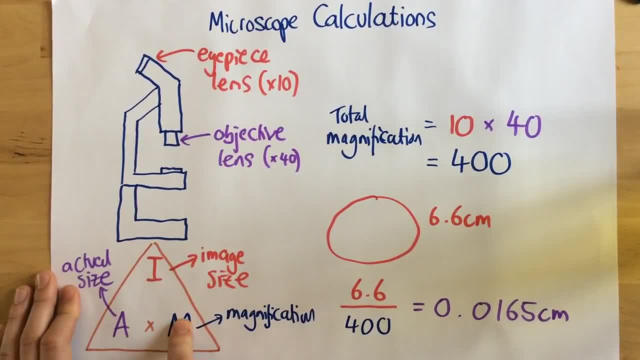 And in order to find the image size, actual size or magnification, you use this equation triangle of: I am. Thank you very much.